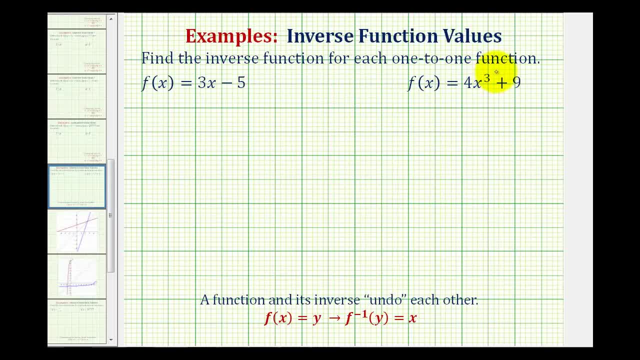 We want to find the inverse function for each of the given one-to-one functions. They're telling us the given functions are one-to-one, so that we know that the inverses are also inverse functions. Remember, functions and inverse functions undo each other. 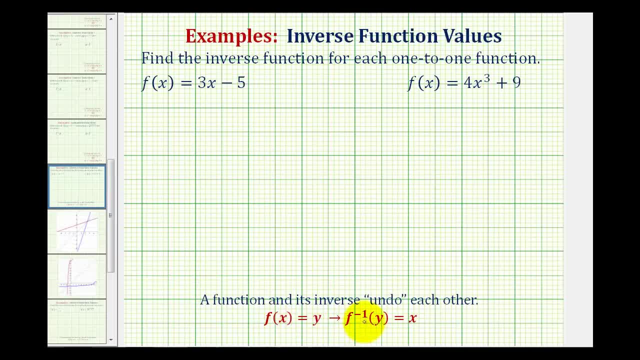 So, for example, if f of x equals y, then f inverse of y would be equal to x. So for every point on the function with an x coordinate of x and a y coordinate of y, the inverse function would contain a point with an x coordinate of y and a y coordinate of x. 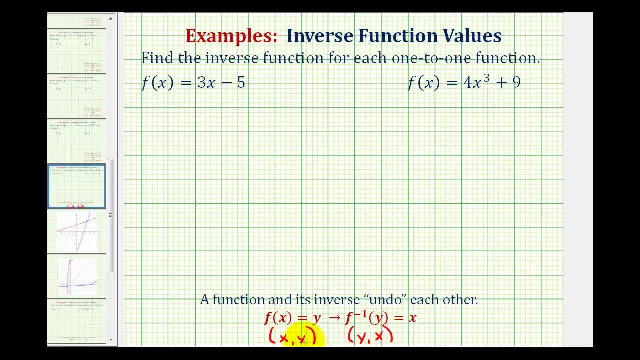 Notice how, if we have a point on a function and we interchange the x and y coordinates, we would find a point on the inverse function, And we can use this idea to help us determine an inverse function given a function. The first step here is going to be to replace f of x with y. 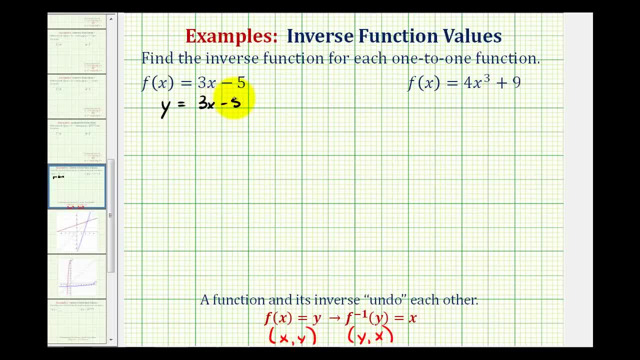 So we have y equals three, x minus five, And then to determine the inverse function, we're going to interchange the x and y variables. So the inverse function would be x equals three, y minus five. But now we do want to solve this for y. 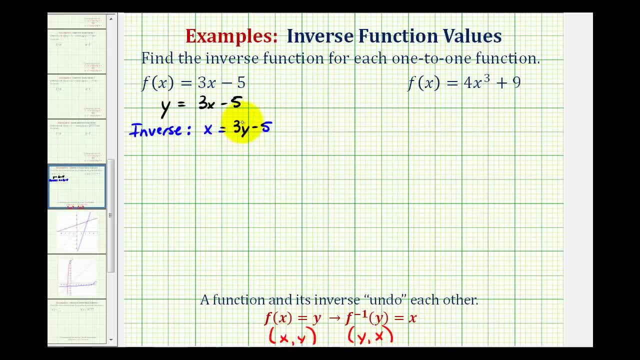 and then replace y with inverse function notation. So to solve this for y we'll start by adding five to both sides of the equation. So on the left, x plus five equals on the right this is zero. so we just have three y. 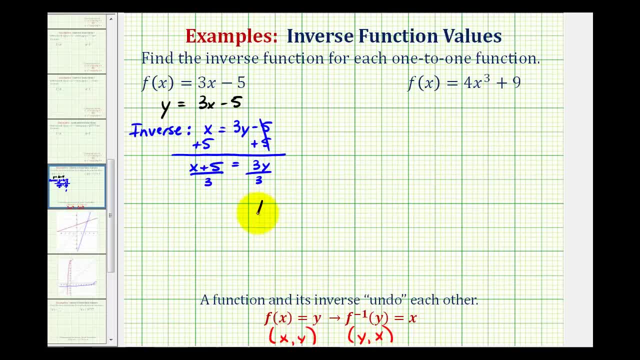 And we divide both sides by three. So we have y equals quantity x plus five divided by three. This is our inverse function. So now we'll replace y with f inverse of x. So f inverse of x is equal to the quantity x plus five. 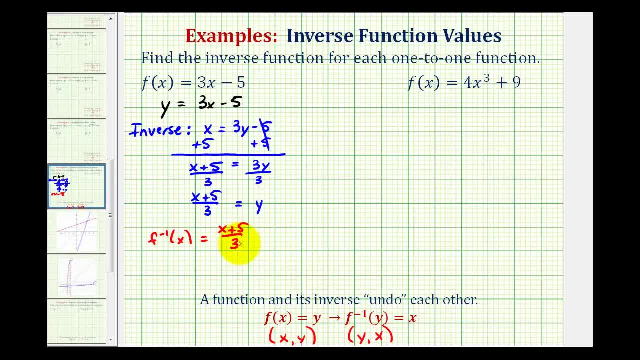 under the x plus five divided by three. Or, if we wanted to, we could write this as two separate fractions. We could write: f inverse of x is equal to x over three plus five over three. Written like this, we can see that the inverse function. 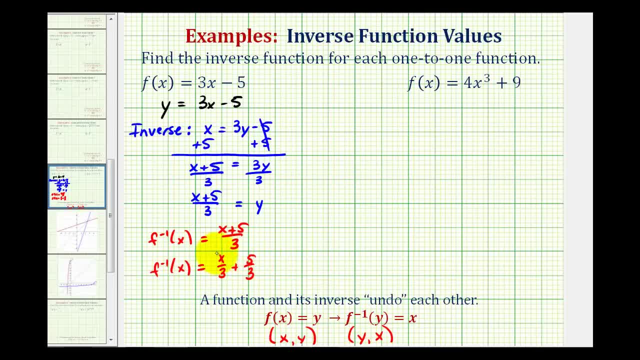 is just a line with a y intercept of five thirds and a slope of one third. And if we do have access to graphing software, there's a nice graphical way to verify that we have found this inverse correctly If we graph the original function and the inverse function. 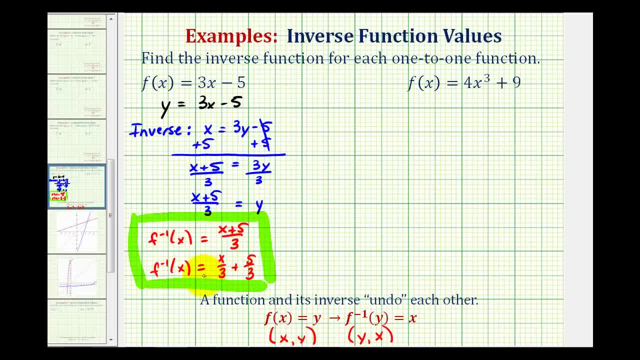 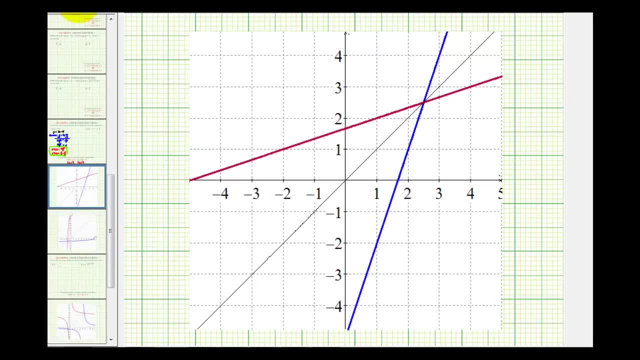 on the same coordinate plane along with the line y equals x. the function and its inverse should be symmetrical across the line y equals x. So, for example, in blue we have the graph of the original function And in red we have the graph of the inverse function. 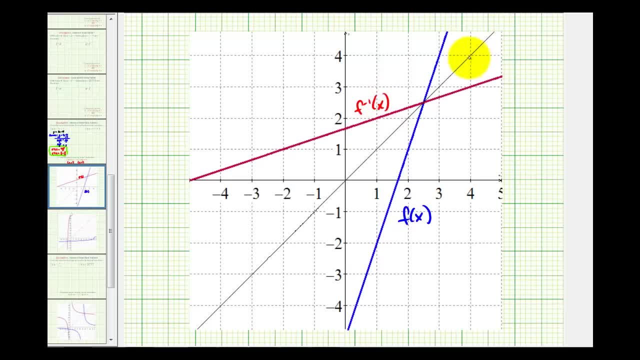 And this thin black line is the line y equals x. Notice how, if we were to fold the line, we would have to fold the line. So if we were to fold these two functions across the line y equals x, they would match up perfectly with the other function. 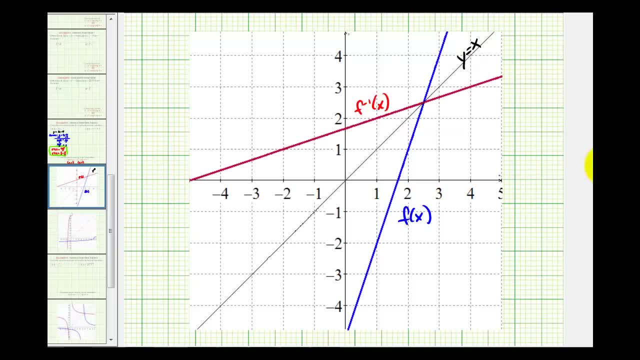 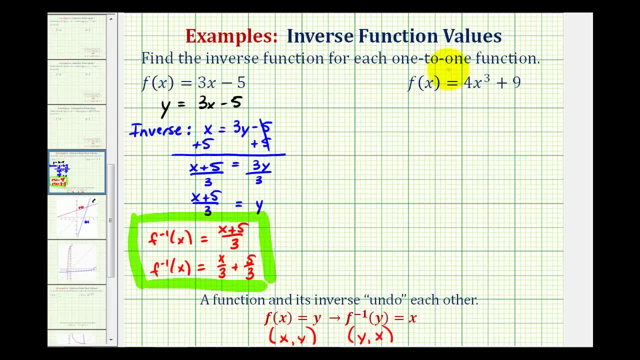 Therefore they're symmetrical across the line. y equals x. verifying, we found the inverse function correctly. Let's take a look at our second example Again. the first step is to replace f of x with y, So we have y equals four x cubed plus nine. 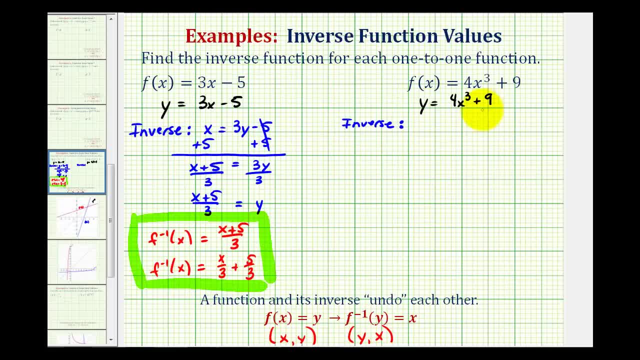 And now to determine the inverse function. we just interchange the x and the y, So the inverse is going to be: x equals four, y cubed plus nine. Again, this is the inverse, but we do want to solve this for y, So we'll start by subtracting nine on both sides. 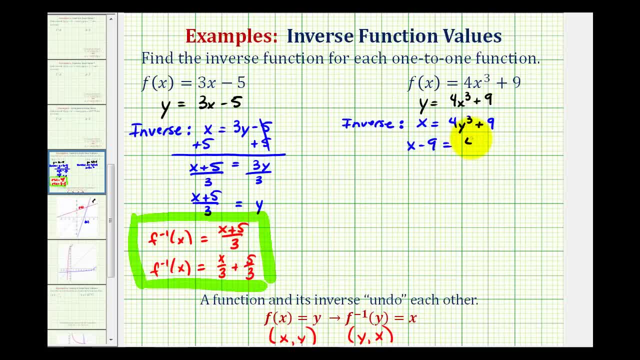 So we'd have x minus nine equals four y cubed Divide both sides by four. So we have y cubed equals the quantity of x. So we're going to have x minus nine equals four y cubed: The quantity x minus nine divided by four. 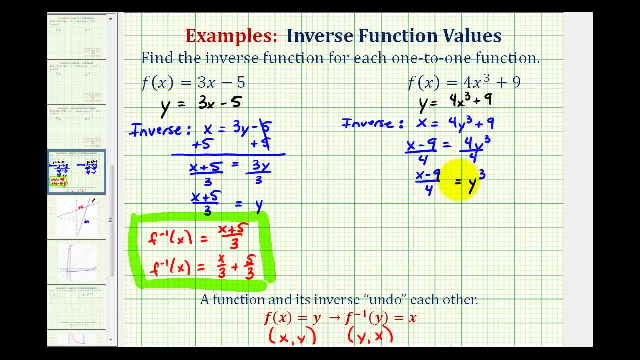 And now to undo this cube, we will cube root both sides of the equation. So on the right side we now have y. On the left side we'd have the cube root of the numerator all over the cube root of four. But if we're required to write the numerator, we're going to have the numerator. 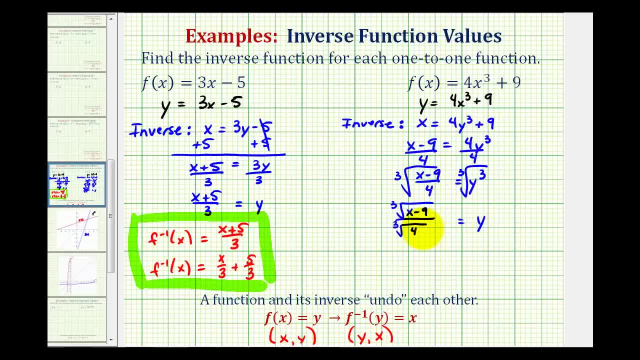 But if we're required to rationalize the denominator, we'd want the denominator to be a perfect cube. And since four is equal to two times two, if we multiply this by the cube root of two, we'd have the cube root of eight, which would simplify perfectly.